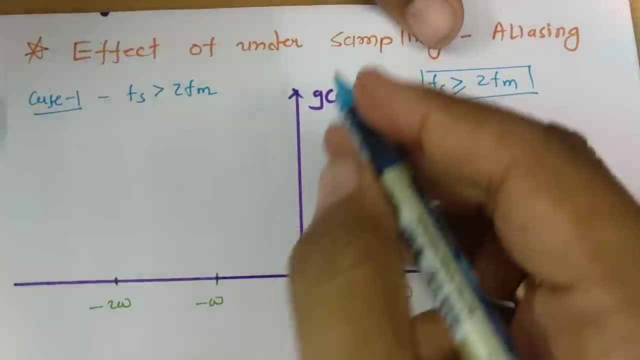 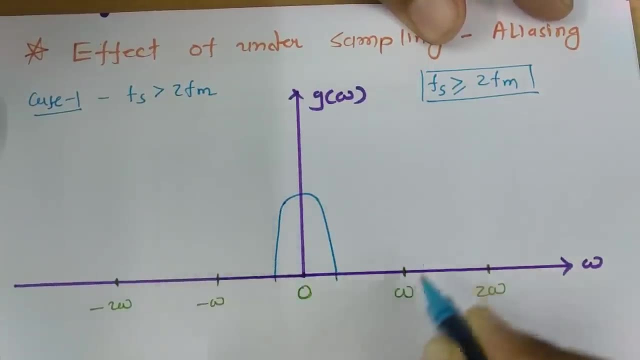 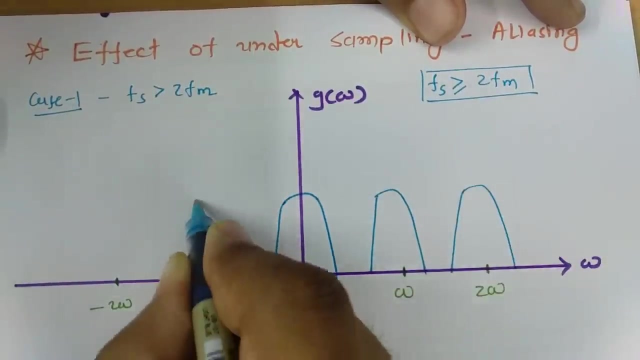 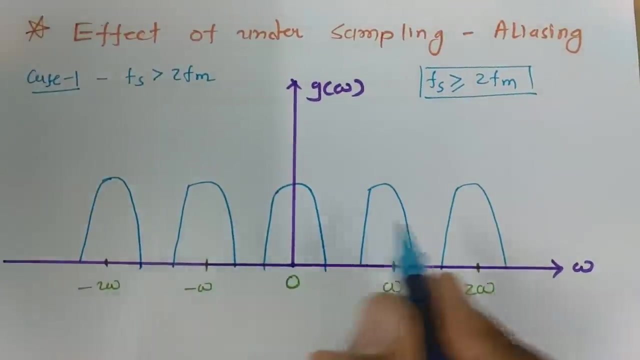 greater than 2fm, Then this is what over sampling. So we can say for this signal response that will be somewhat this, So you'll be finding there is no overlapping of responses. So this is our response will come if Fs is greater than 2fm. Now, 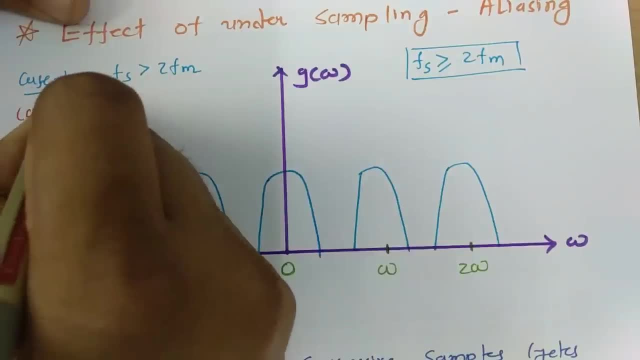 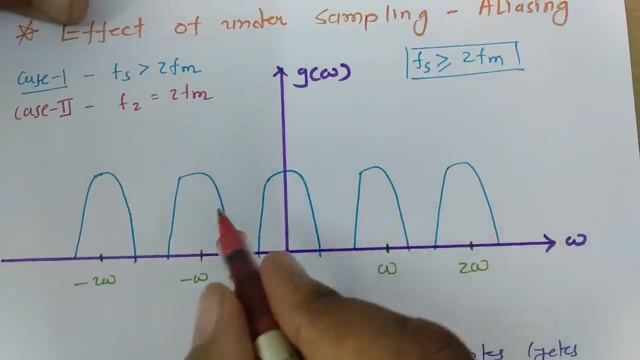 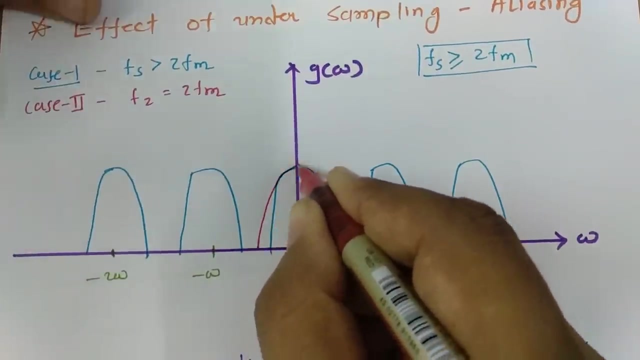 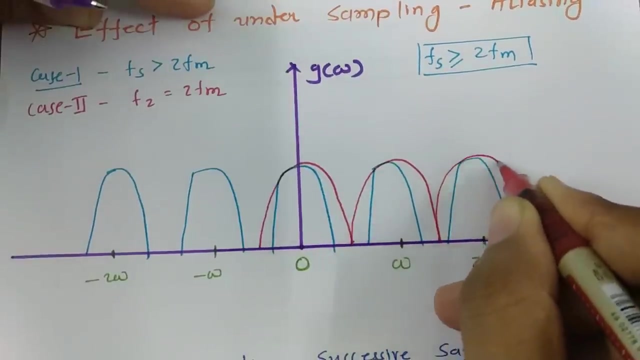 if we consider second case, that is, Fs is equal to 2fm. So in that case, this samples of frequency that will just touch to each other, So you'll be finding response will be somewhat this: This samples will just touch to each other like this And so on. there will be continuous. 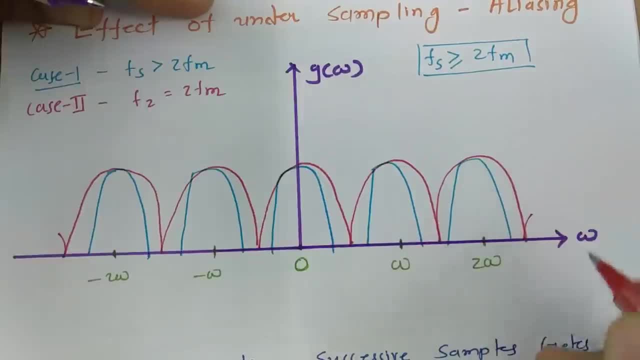 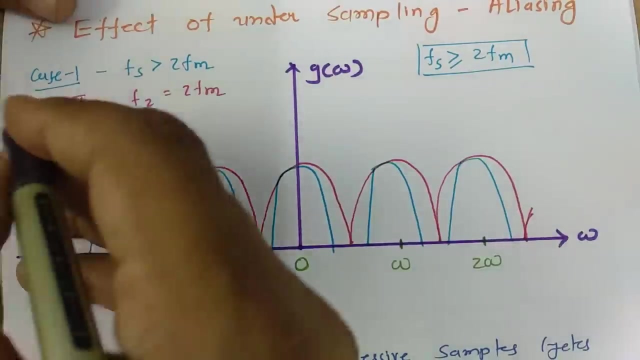 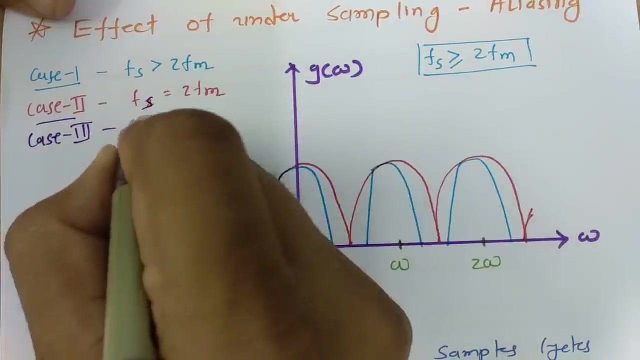 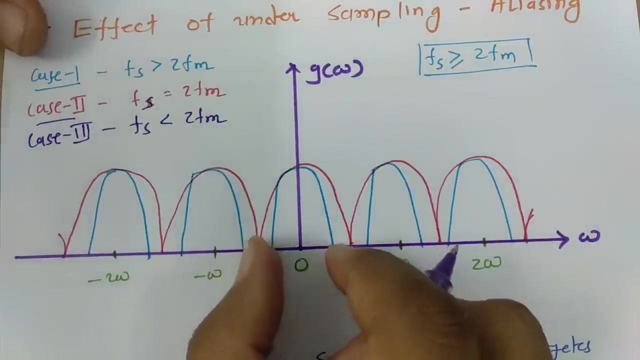 infinite samples. So it will be continuous up to infinite frequency. Now if I consider third case, So for third case, this is what: under sampling, What if Fs is less than 2fm? So see here what happens: This frequency, Fm Now that is increasing, like this, So as if frequency increases consecutive. 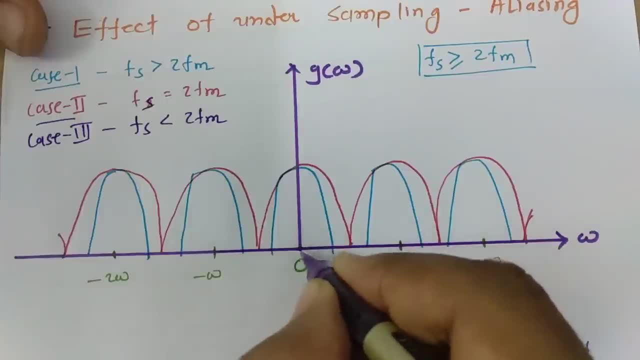 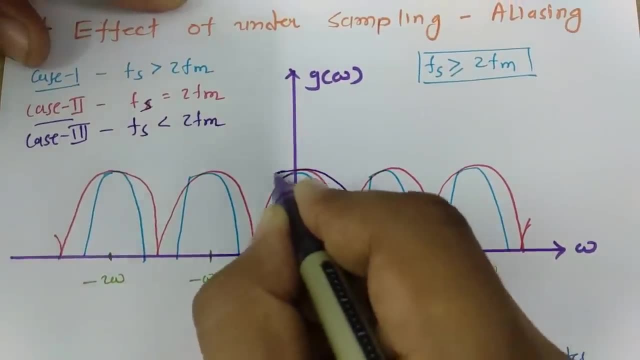 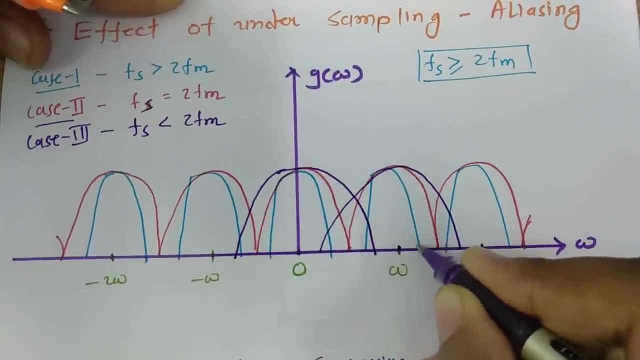 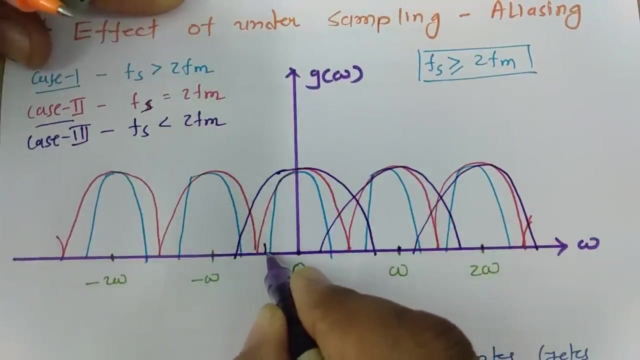 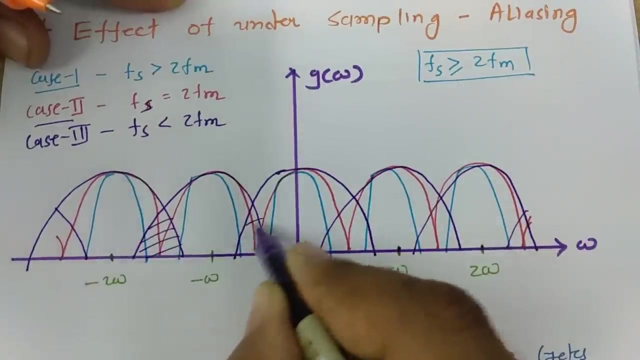 samples will overlap to each other. So see for this: up to f, omega m. if it increases up to this like this, One can see for this, even you'll be finding it increases like this For this, it will increase like this, Similarly on negative side. So here one can see This is where there is overlapping. 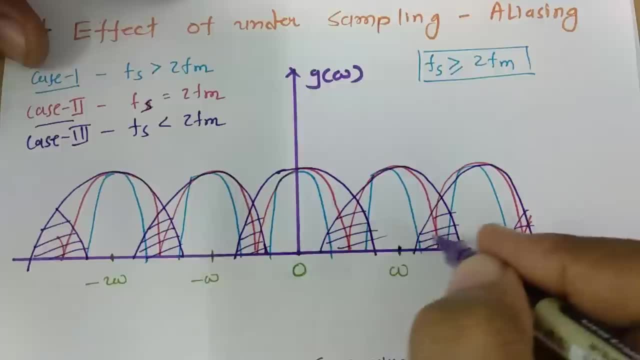 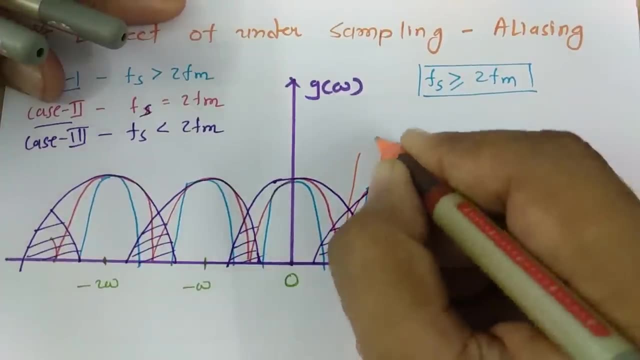 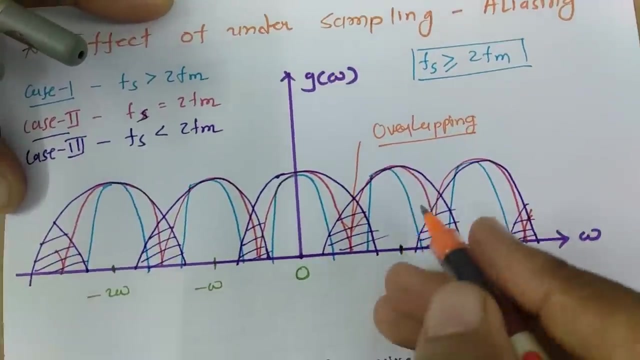 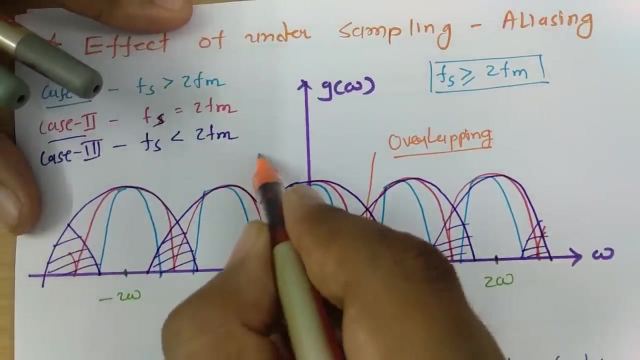 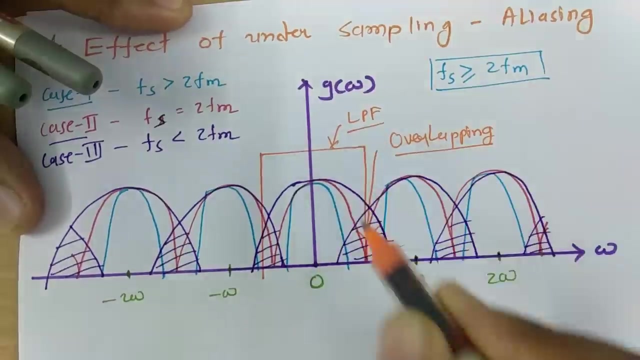 This is where there is overlapping. So, because of this overlapping, Because of this overlapping, When you use low pass filter to extract original information, there will be distortion. The reason is you just place over low pass filter like this and try to extract information. 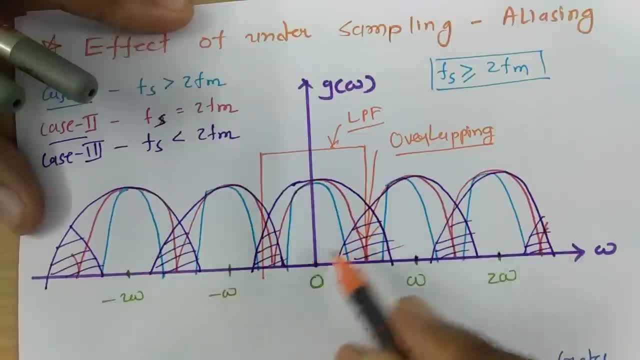 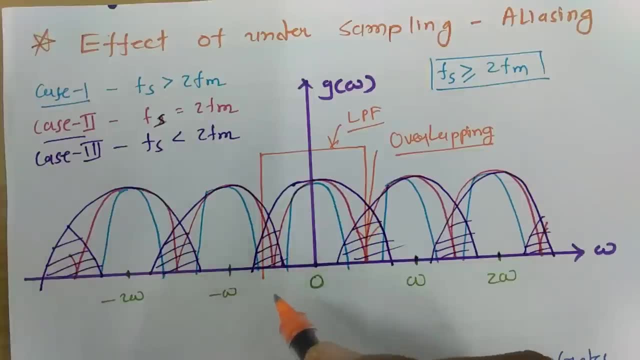 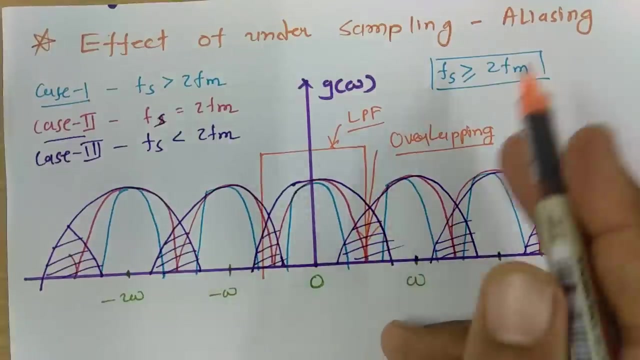 So there will be information of this sample as well as this sample Right, So you cannot extract proper signal. The reason is it will be mixture of two different signals, So there will be a possibility of distortion. So this is what allysing. So because 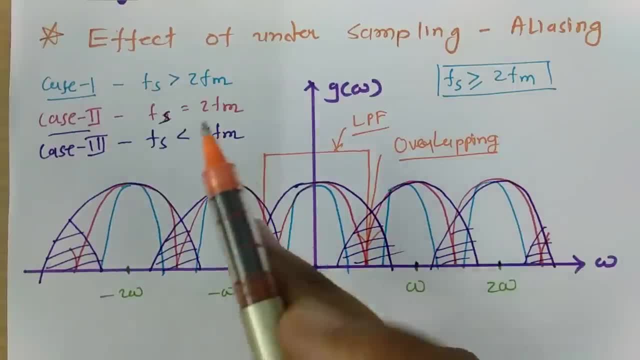 of allysing, overlapping is happening and that happens in case of Fs is less than 2fm. that is even referred as under sampling. So if Fs is less than 2fm, it is under sampling At the time there will be overlapping of consecutive 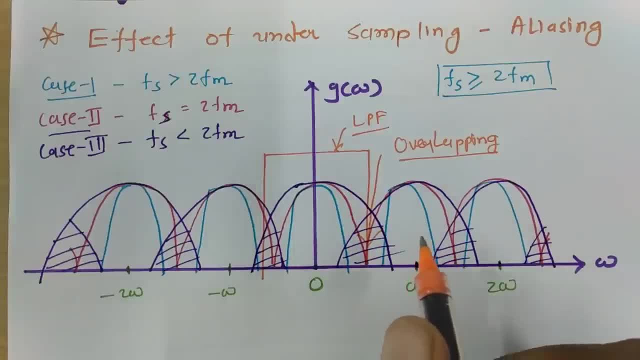 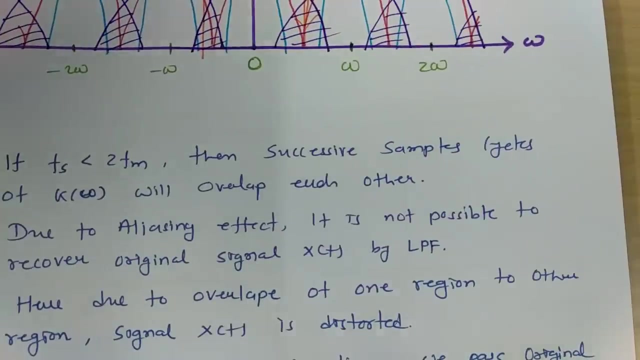 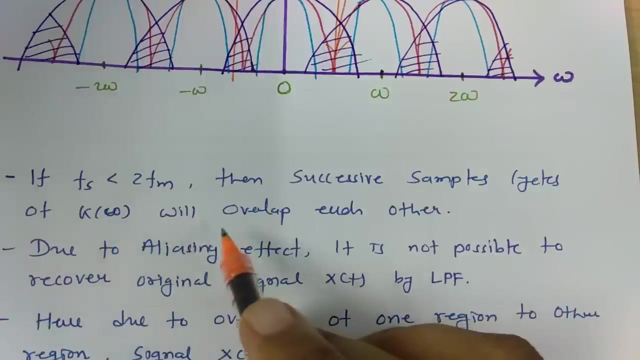 Samples of frequency response and because of that there will be distortion when you extract signal by passing through low pass filter. So this is what the basic problem that will happen. Now see, if Fs is less than 2fm, then successive sample cycles of Gf Gomega will overlap each other. That we have seen already, Due to allysing effect. 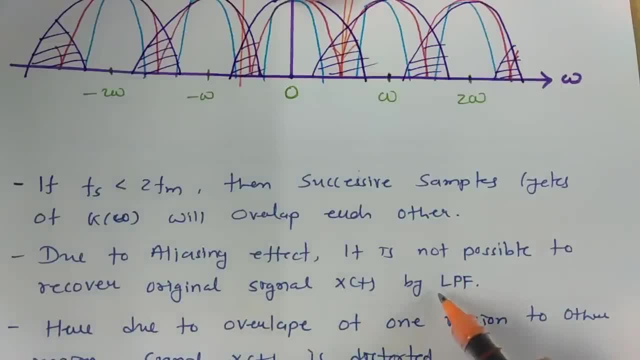 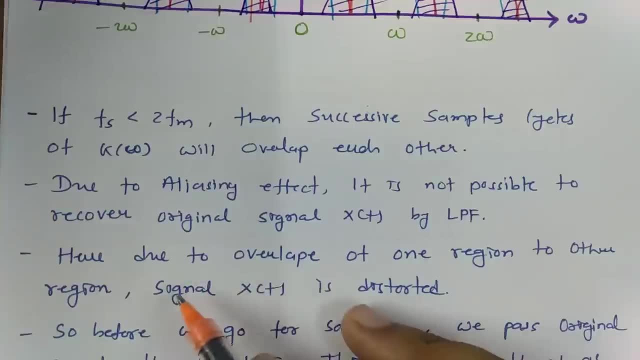 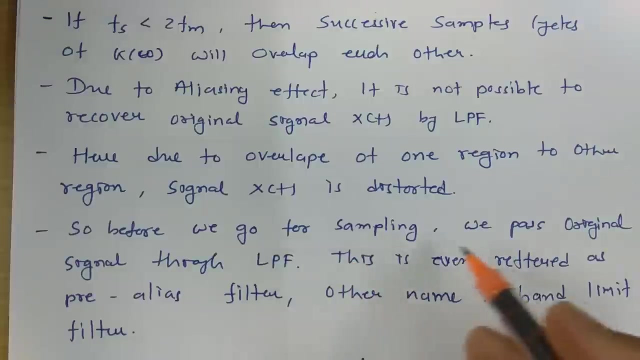 It is not possible to recover original signal Xt by low pass filter Here due to overlap in one region to other region, signal Xt that is distorted. So before we go for sampling, if we pass original signal through low pass filter, that is even referred as pre allysed. 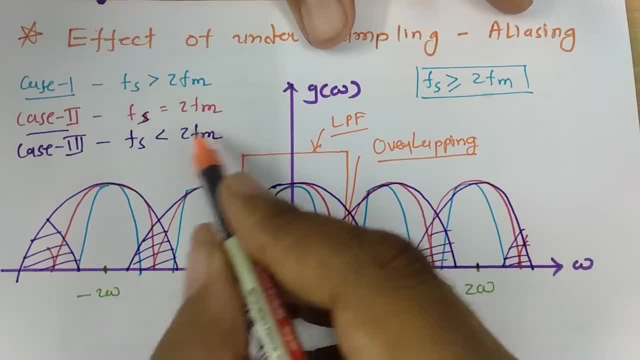 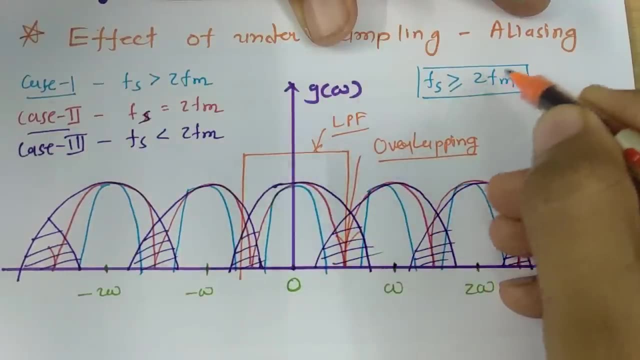 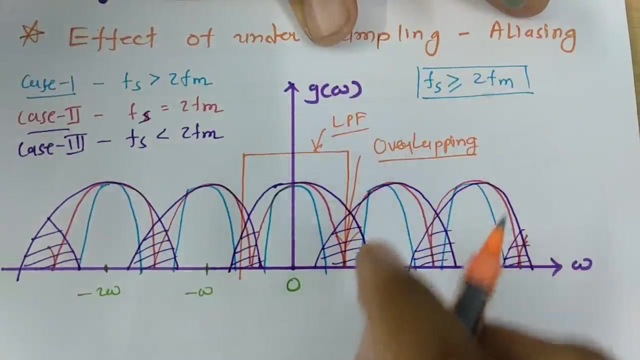 filter. So see if we keep our Fm Smaller. In that case we can provide this condition. So if Fm is small, Then we can have satisfaction of this condition, Like see, for example, if our Fm is big. in that case